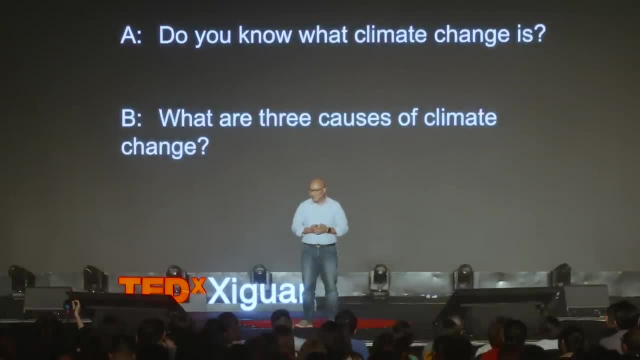 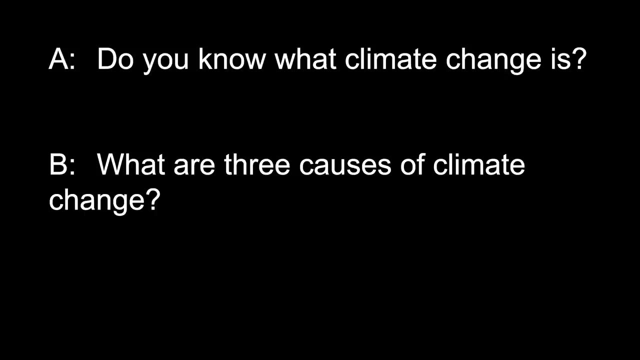 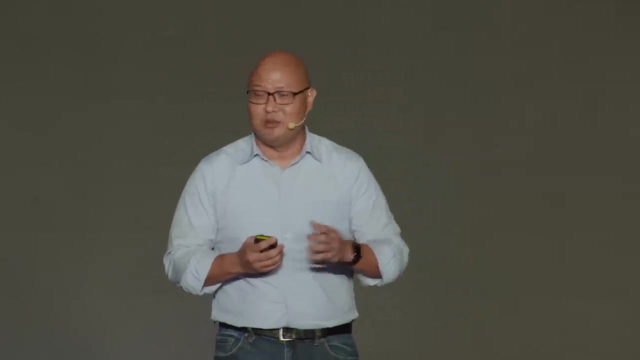 Do you know what climate change is? And the second one, question B, reads: What are three causes of climate change? Now, which one of these questions better assesses student learning? If you said B, you're right. Question B requires you to possess a specific type of knowledge in order to answer this question. 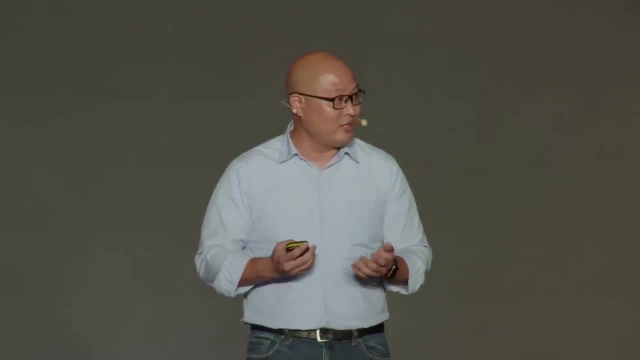 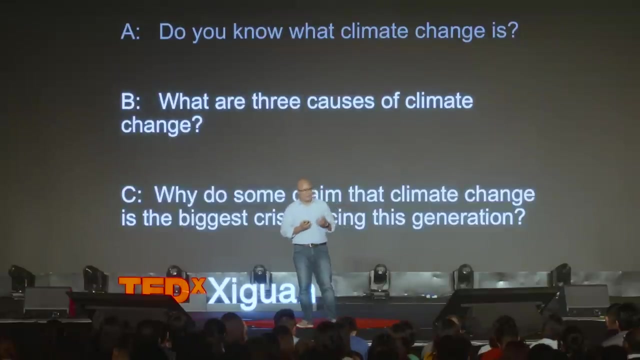 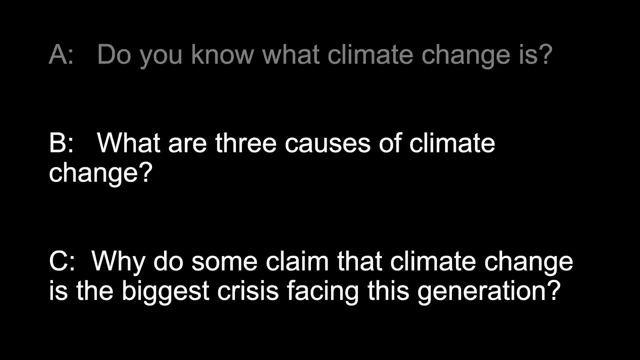 Either you have this information or you don't, And so let's go ahead, and this time we'll add another question into the mix. Take a look at question C. Why do some claim that climate change is the biggest crisis facing this generation? Now, which one of these better assesses student learning? 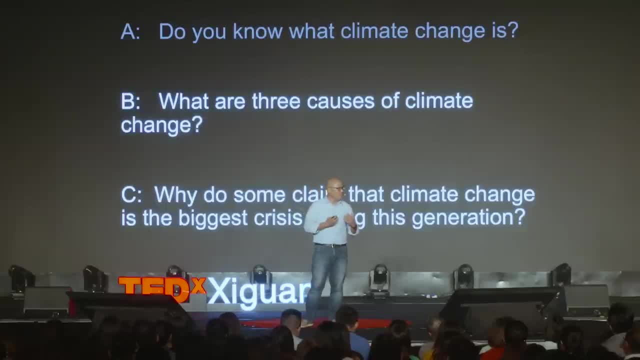 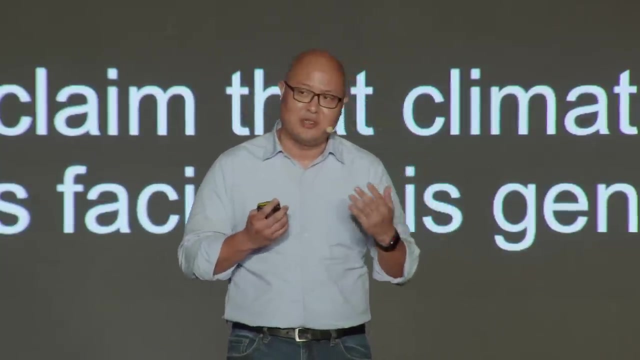 Well, this question may be a little more difficult than the previous one, because they both can, And so the former assesses student knowledge, while the latter gives students an opportunity to think of the consequences of an impending disaster. And so, in the ideal class, students would first ask, or teachers rather would first ask question B to establish the foundation knowledge. 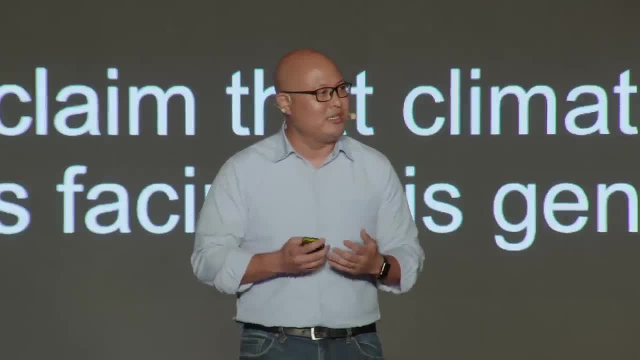 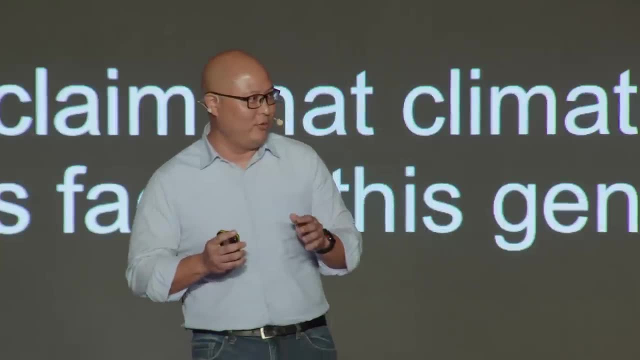 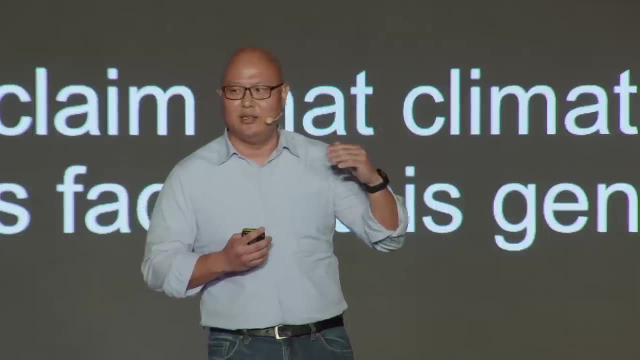 And then they would ask question C to give students an opportunity to use this knowledge. Now think back to when you guys were kids, When you guys were in school, And I know for many of us this may be a difficult, painful experience. But think for a second. if your teacher only asked you questions like question B, 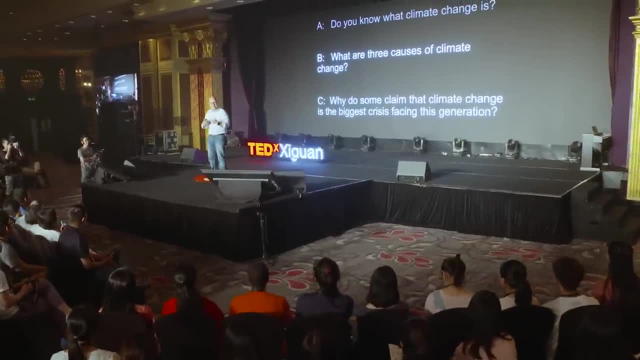 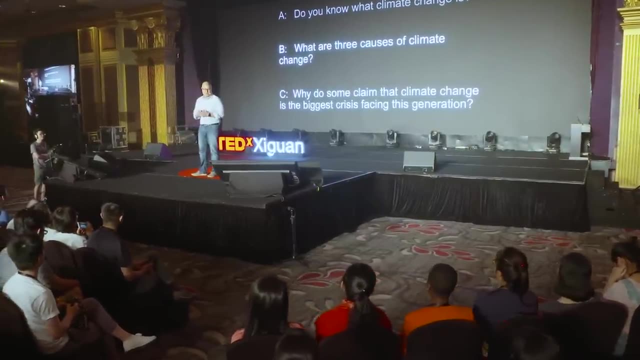 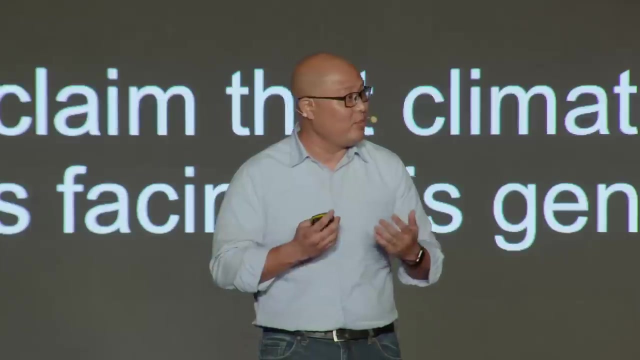 Well, this might be great for trivia contests, But we would never get an opportunity to use or put this knowledge to good use And think about for a second, if your teacher only asked you questions like question C, and these are pretty difficult questions. 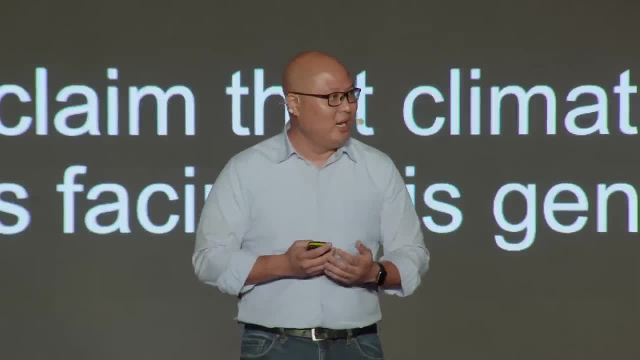 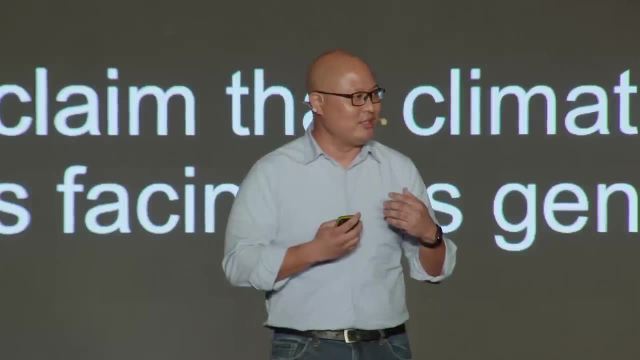 This might serve to frustrate your learning and maybe you'd be tempted to give up before you even get started. Now back to the observations. I went on these teacher observations recently and we saw different classes, but I noticed that there was something in particular that was lacking. 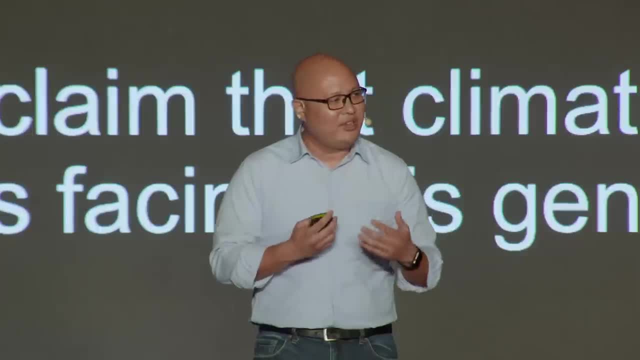 And while the teachers were certainly well-prepared and there was a lot of engagement going on in the classes, an overwhelming 90% of the questions that were asked were of lower-order question types. In other words, they looked more like question B. 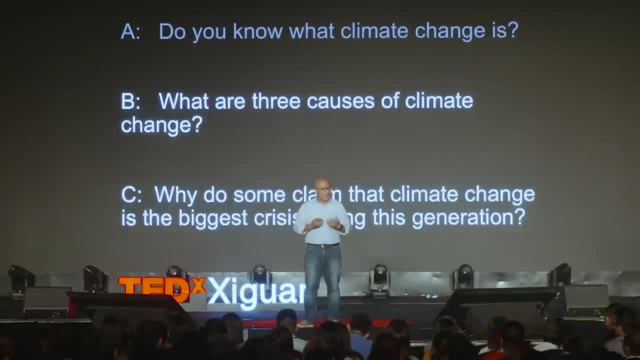 And in three of those classes, not one single higher-order question was even asked. And so how does this even happen? Well, asking higher-order questions is the key to stimulating critical thinking, And we need to be able to give students an opportunity. 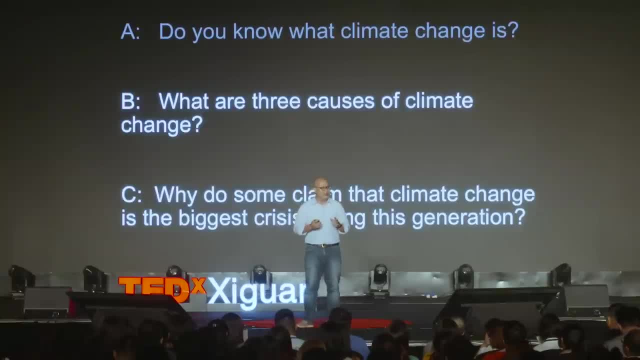 to grapple with questions that don't necessarily have one correct answer. This is more realistic of the types of situations that they're likely to face when they get outside of the classroom. Now, teachers shouldn't have to bear the responsibility on their own. 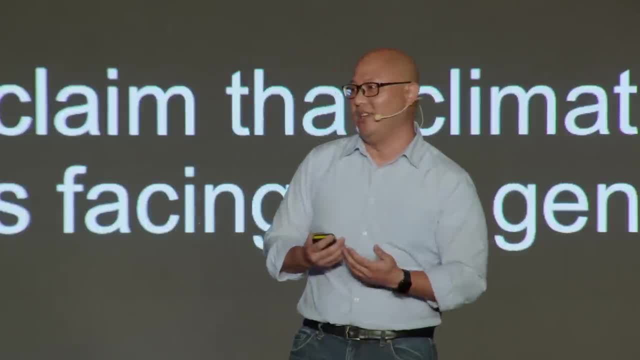 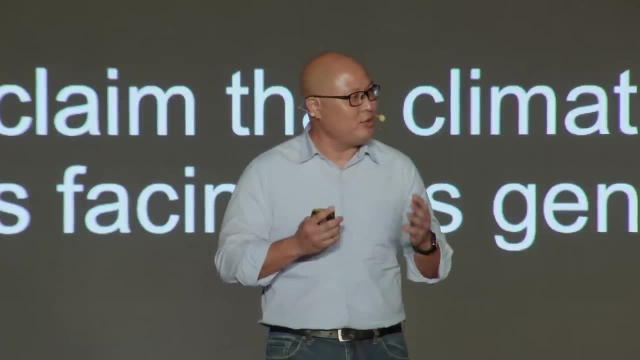 When it comes to something as important as critical thinking, then it's all of our collective responsibility in order to push students forward. In other words, when it comes to creativity, the door doesn't just shut when the school day ends, And as the parent of school children myself, 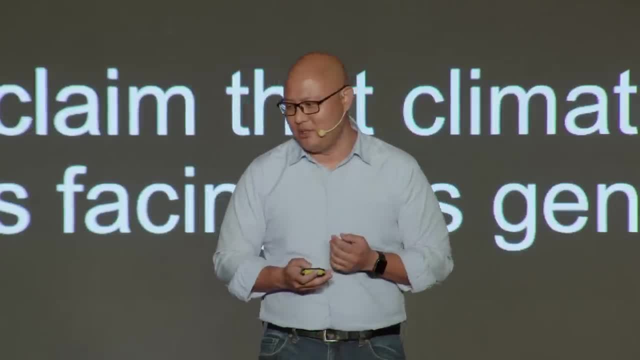 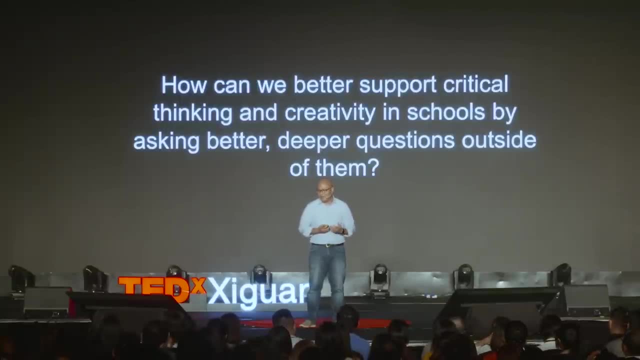 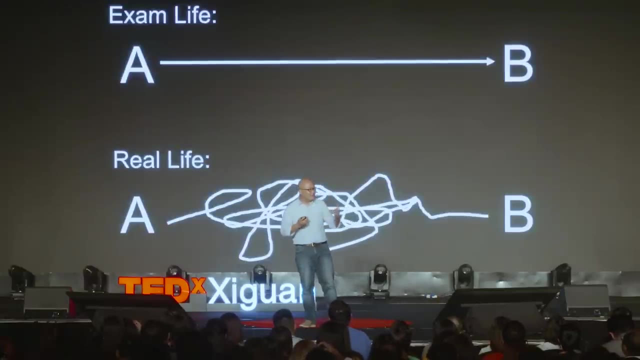 it got me thinking about the following question: How can we better support critical thinking and creativity in schools by asking better, deeper questions outside of them? Now, as we know, we can study easier questions, we can answer easier questions, and this is great for exams. 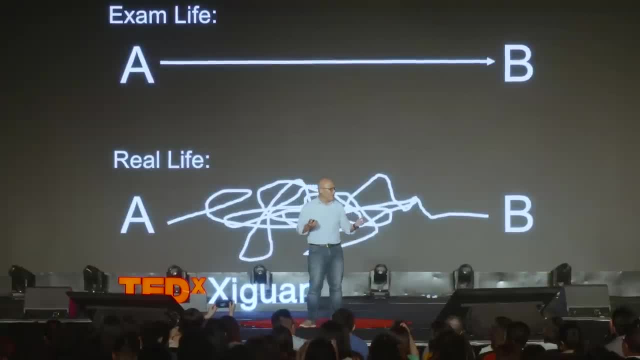 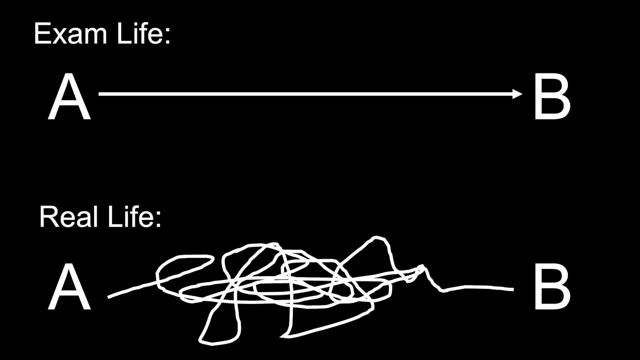 But as participants in society, we all know that we have to deal with questions that are a lot more complicated than those found on a multiple-choice test. In reality, right, and we can see here, real life is a bunch of squiggles. 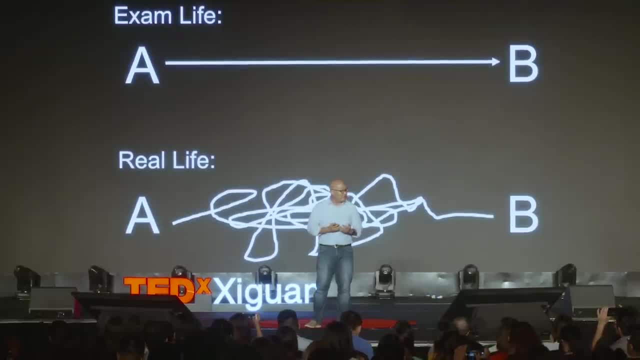 There is not necessarily a blueprint that tells us how to get from A to B, And so, with this type of situation, it's important that we expose our students to a degree of uncertainty in their classes, and not just wait until they have to experience it for themselves. 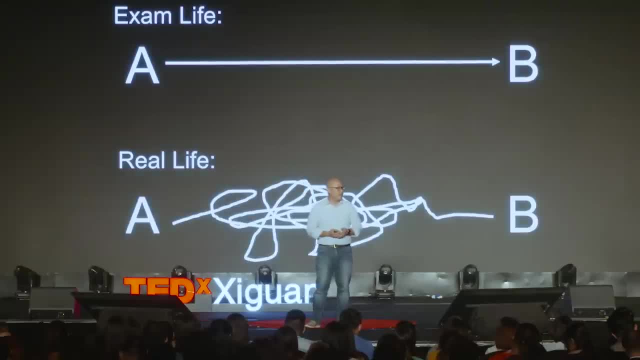 for the first time outside of the classroom. You know, these days we send our kids to piano practice at age four, maybe soccer practice at age five. maybe they learn English at three months, I don't know. it's getting earlier and earlier. 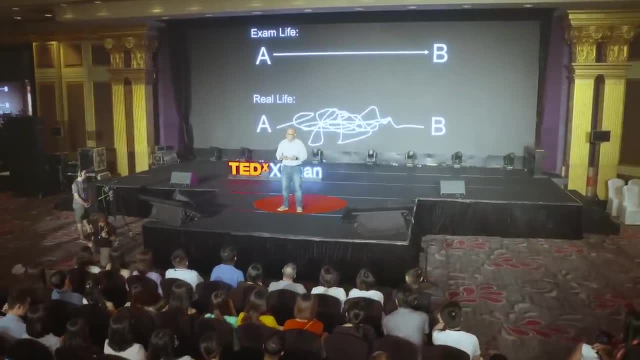 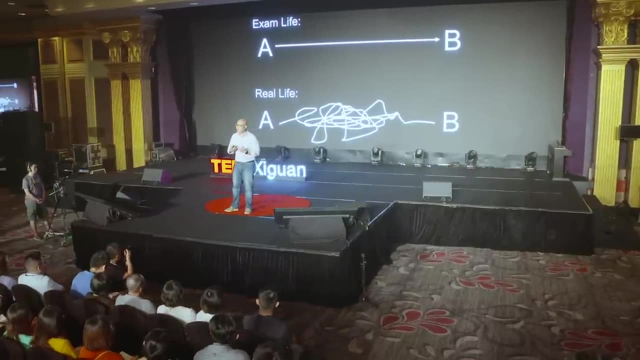 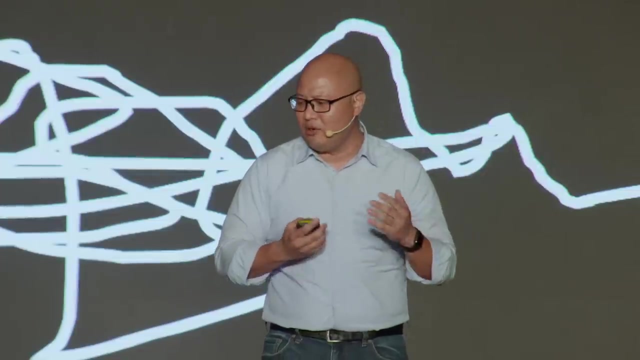 But one of the reasons why we do this is to give students an opportunity to learn some subjects or to be exposed to things that they normally wouldn't be able to do outside of the classroom. So when it's something as important as critical thinking at stake, 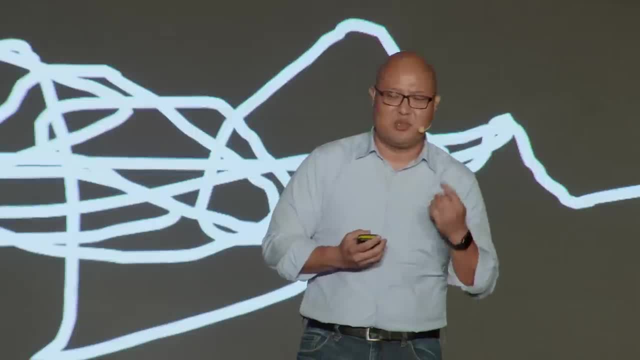 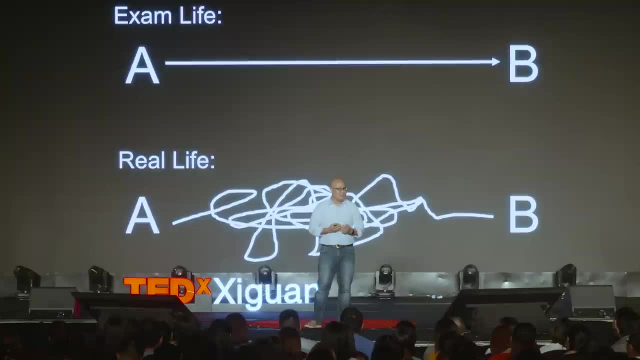 does it not also make sense to expose our students to these tougher questions earlier, when the stakes are not as high? Now, let's think about this. Now, when we ask tougher questions, such as why questions, it's a lot more difficult. 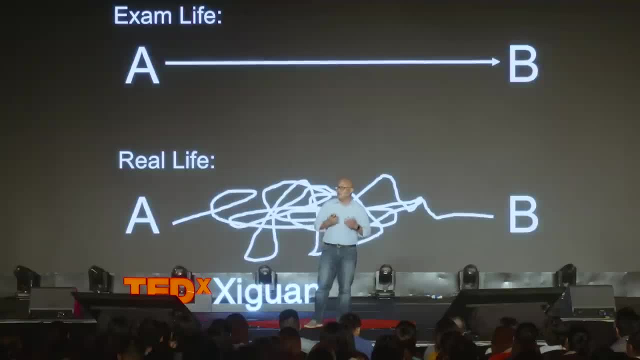 And it's difficult for a number of different reasons, And one reason it tends to be difficult is that, in answering a why question, students need to put themselves out there. There's a risk there. There's a risk that, well, maybe they feel they won't say the right thing. 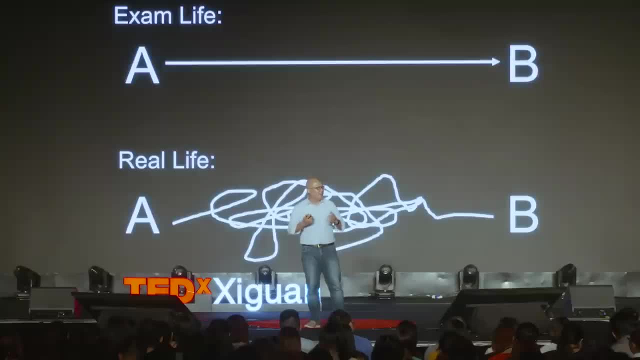 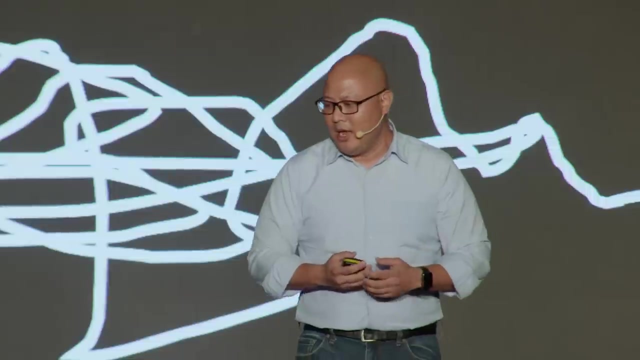 or maybe they'll be judged by their classmates, But we need to do a better job of encouraging this and instilling in our students the grit necessary to be able to persevere against challenging topics that come their way. And so what schools need to then do a better job of. 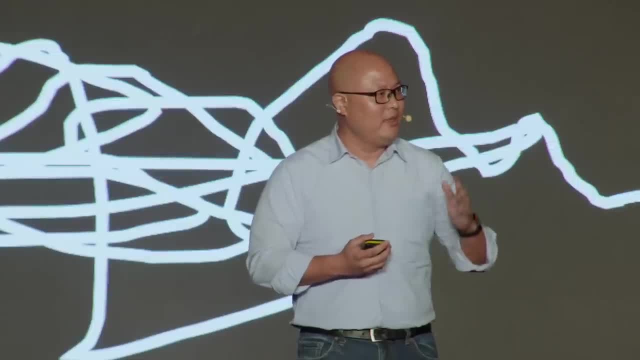 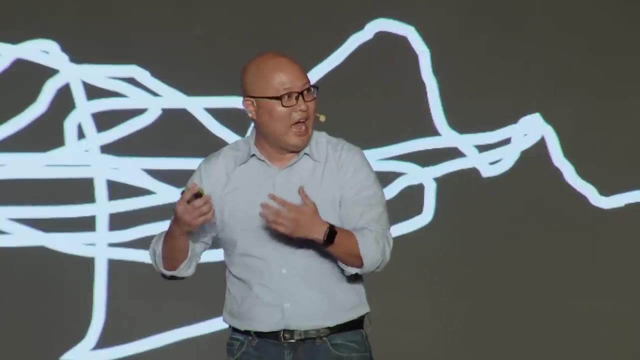 because we assume to a certain degree that in school, students are able to connect the dots for themselves. In other words, we assume that they can take whatever knowledge that they learn in school and somehow be able to figure out how to use it outside of it. 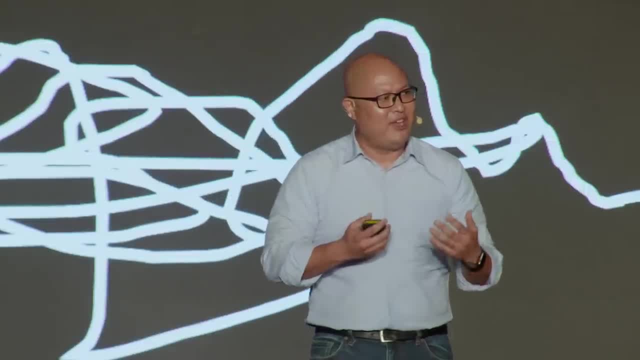 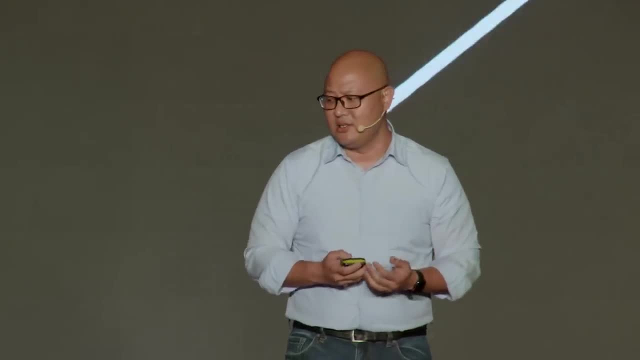 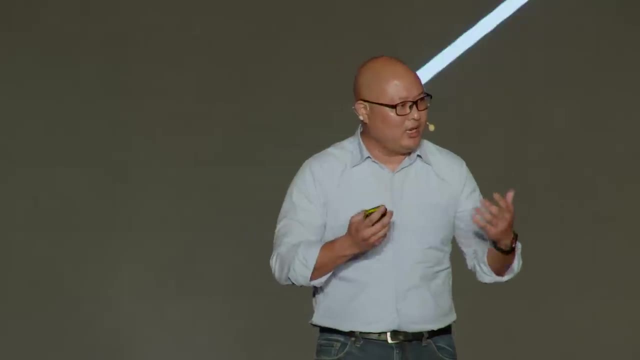 But this assumption is dead wrong And in fact, schools need to do a better job of not just teaching students the what or the contents, but getting them to how, by asking more whys, And luckily we all can play a role in this. 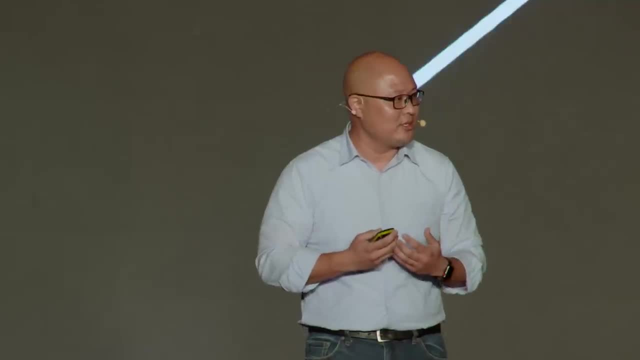 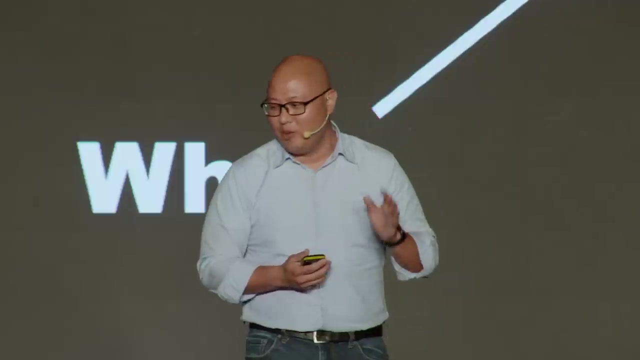 In fact, we can ask better questions by inviting others to ask better questions of us, And here are three ways in which you can do that. So let's go ahead and start with number one. We can first start with a what question, but don't end there. 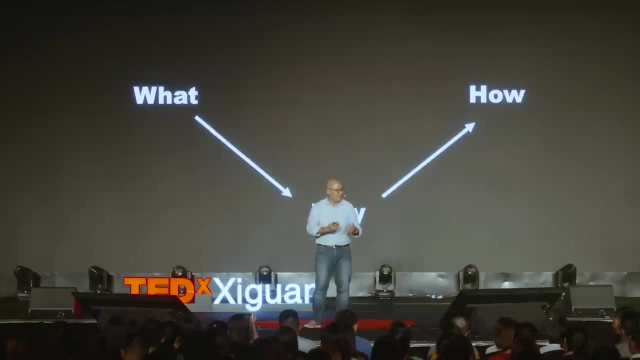 Remember, when we ask a what question, this is the starting point. And when we ask these types of questions in class, students get a little bit excited because it's one of these answers where if you get it, you get it, And if you don't, you don't. 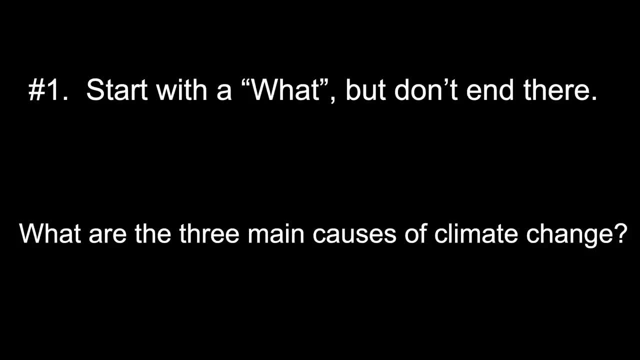 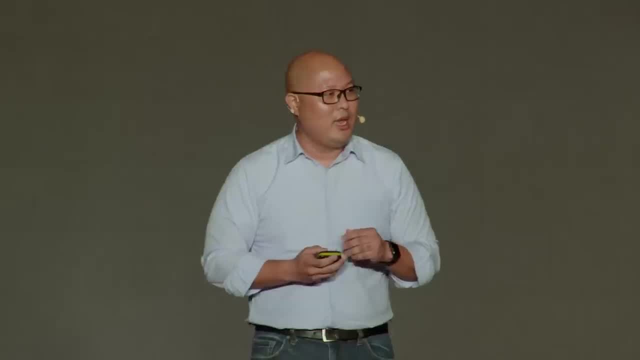 But let's take a question that we started out with earlier, And it's this one: What are three main causes of climate change? And so if I were to ask this to my students, students could easily find the answer by doing a quick search on the internet. 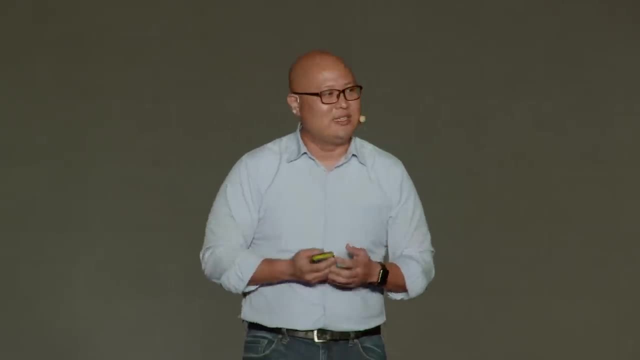 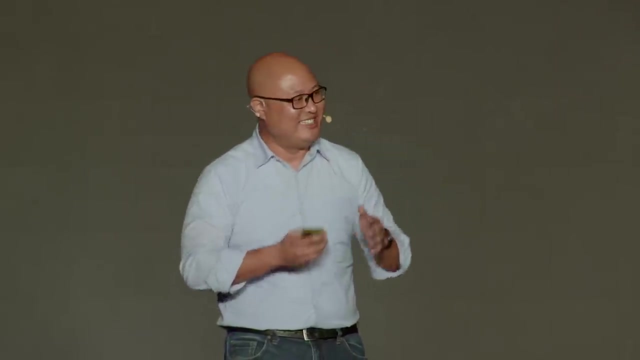 or maybe they would review their class notes. But the point is it would take little effort to answer this type of question. But asking this type of question is deceptive because if you get enough of these right, it could give you this false sense of security. 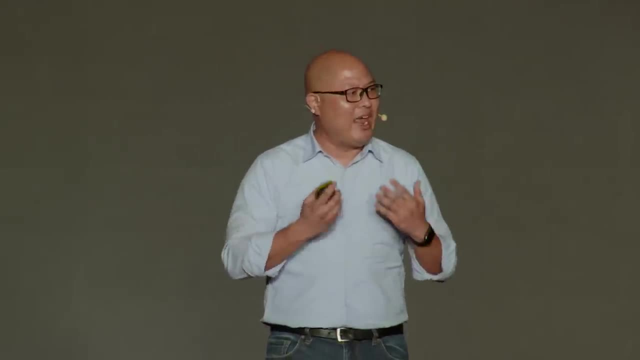 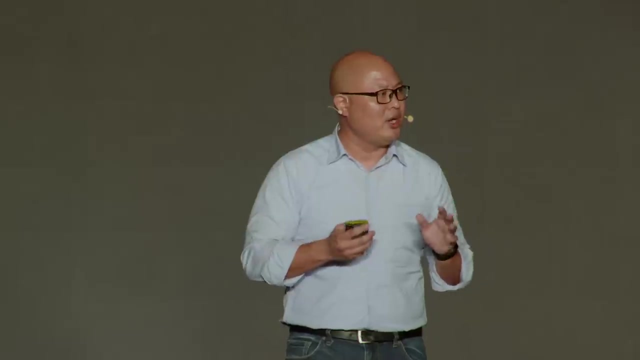 Like: oh, I know the answer right, But, as we know, our jobs in all of this is to move beyond the textbooks, because this is what the textbooks are for, And our job is to put some kind of real-world spin on the type of content that students are learning in school. 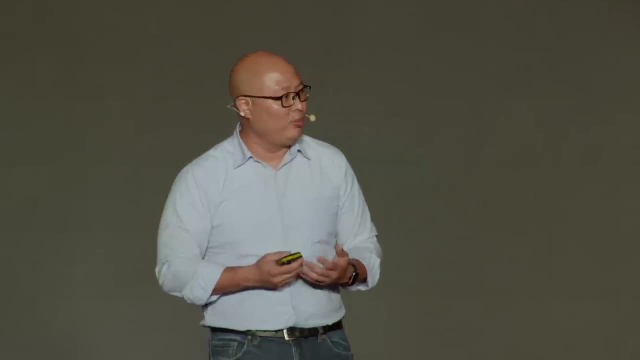 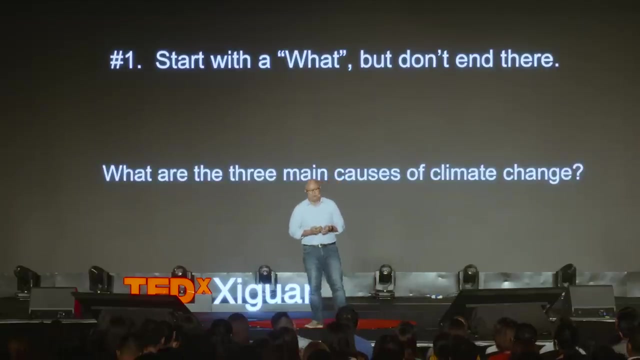 So there's a way to make this kind of question a little more productive. Rather than just asking students the what, what we could do instead is have them explain or paraphrase what they learned in class, And so consider the transformation We changed. what are three causes of climate change? 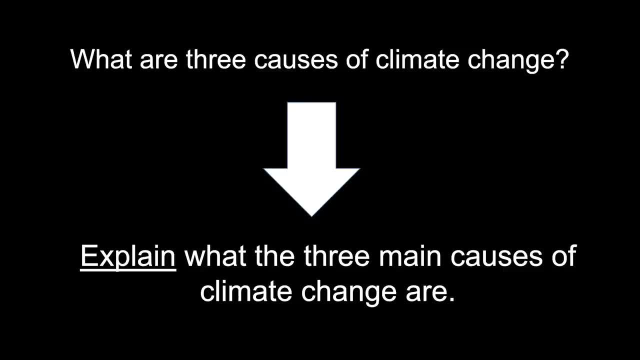 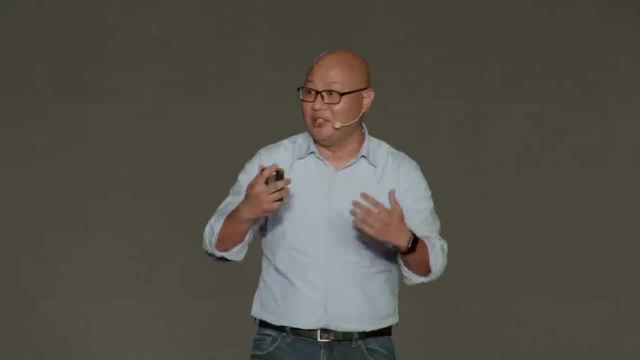 to explain what the three main causes of climate change are, And here, by asking this question instead, students need to give a little bit more. In other words, it's not just a safe answer. They have to go ahead and take that risk. 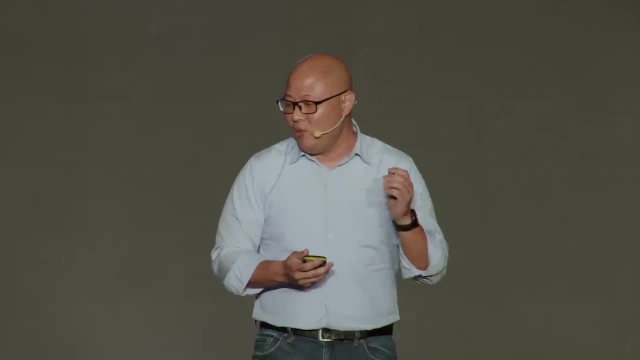 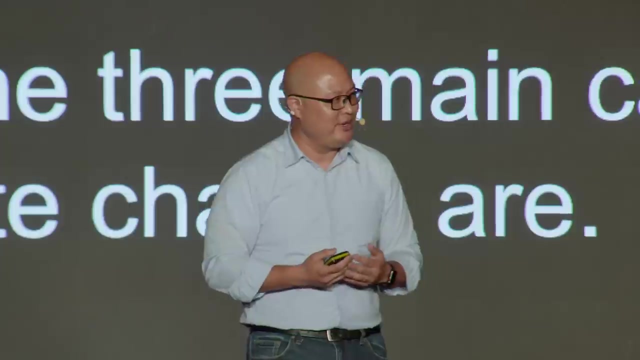 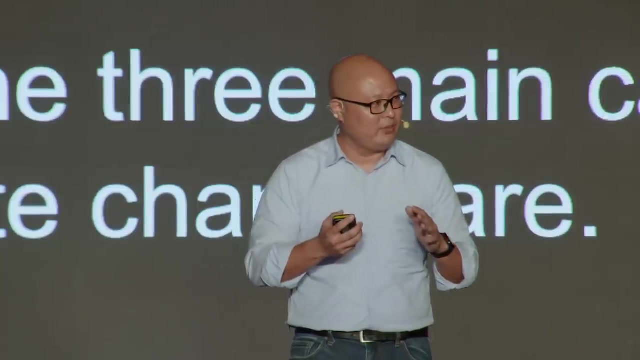 and put themselves out there. So once we've established the what, then we can start making connections by asking a series of why questions. And so asking these why questions gives students an opportunity to connect whatever knowledge they have to something personal in their lives. 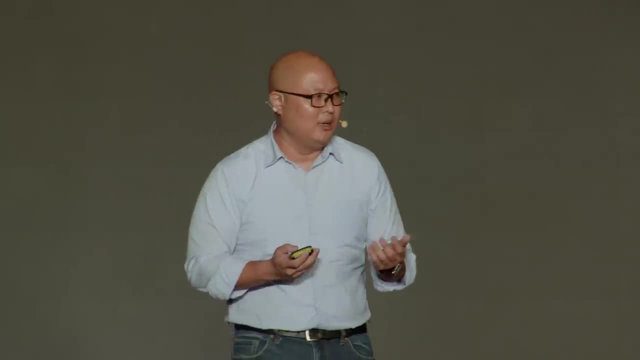 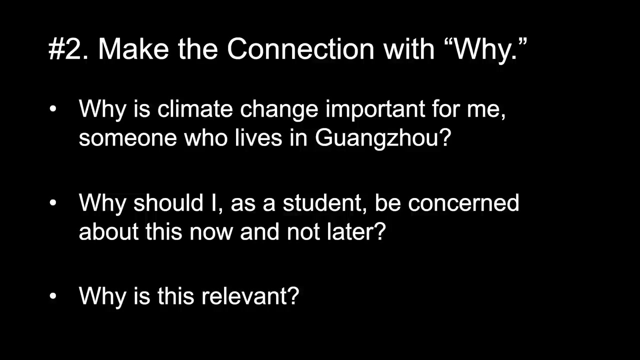 And so here are just some examples of possible why? questions that students can ask. Well, why is climate change important for me, someone who lives here in Guangzhou? Why should I, as a student, be concerned about this now and not later, And why is this relevant? 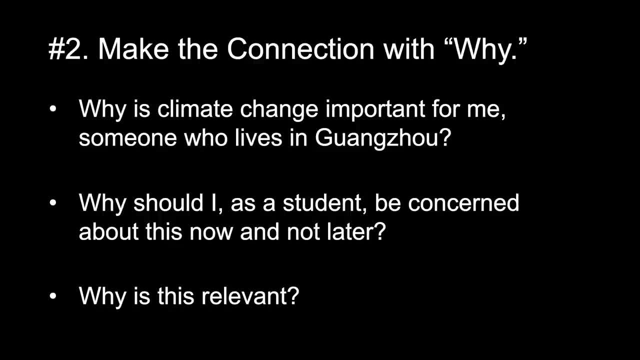 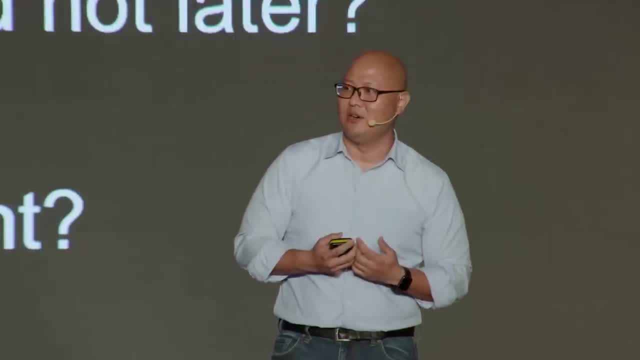 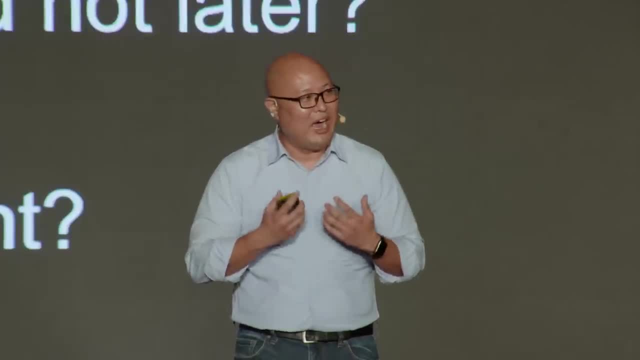 And when students make information or abstract information from textbooks relevant, then they can see the value in this and they start asking themselves, OK, how can I take this information and put it in my sphere of influence? and to think about how this could be useful. 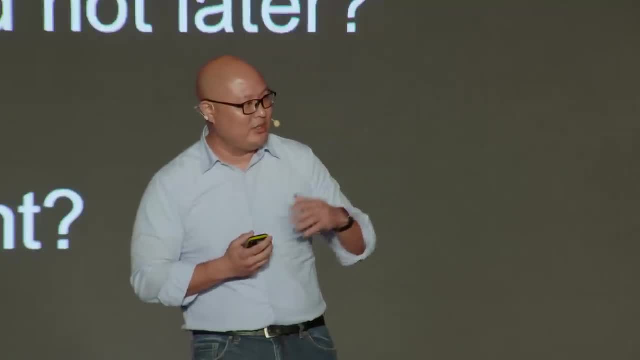 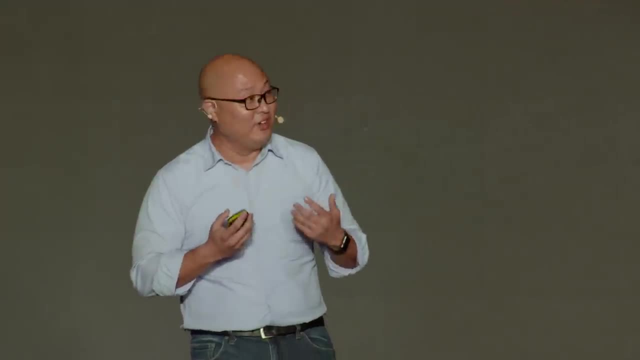 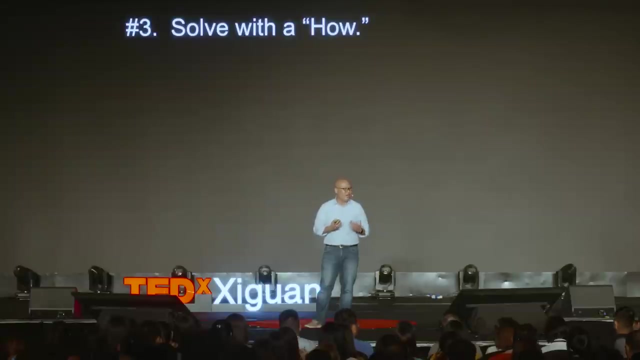 in my everyday life. So once we've established the what and then we've figured out how to connect it with the why, then we can start the fun stuff right, Trying to solve by asking the hows. And here are some of my favorite how questions: 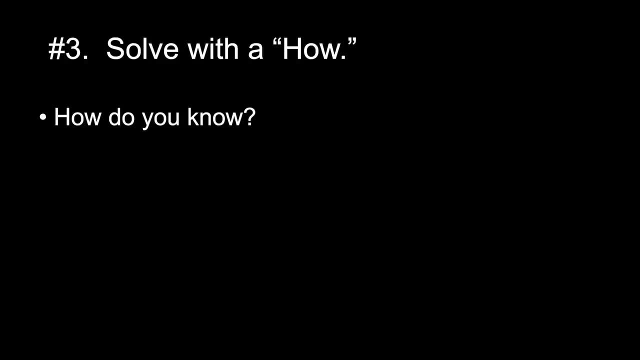 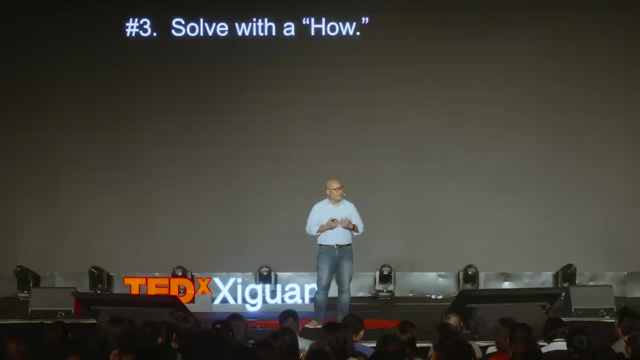 that I like to ask. The first one is: how do you know? So in our earlier question about climate change, rather than just giving the answers, students then have to back up their answers. So what are the three main causes of climate change? 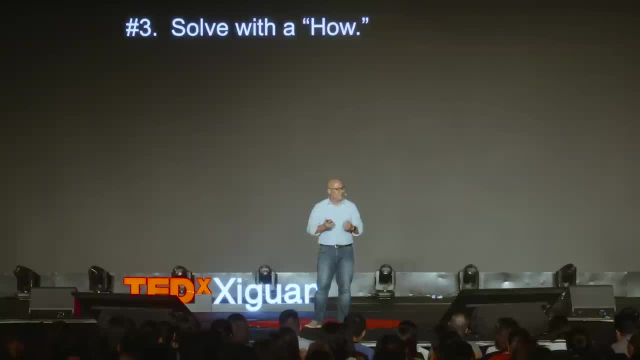 blah, blah blah. and then you can ask: well, how do you know this? And by asking this question, students then cannot just get away with the easy answer. In other words, they have to provide some sort of evidence and to be able to defend their answer. 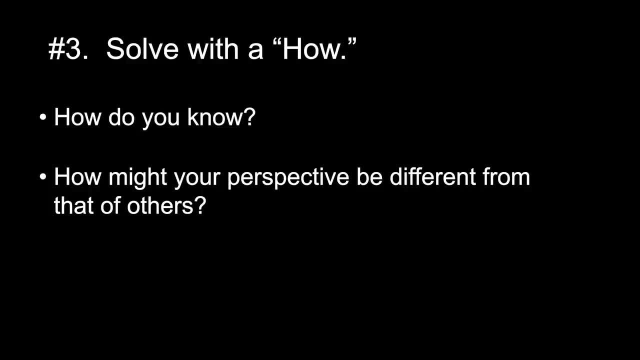 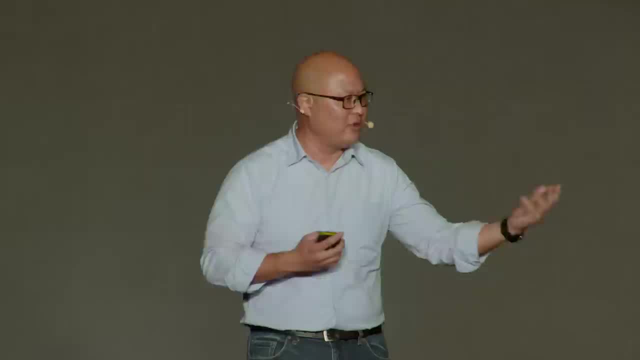 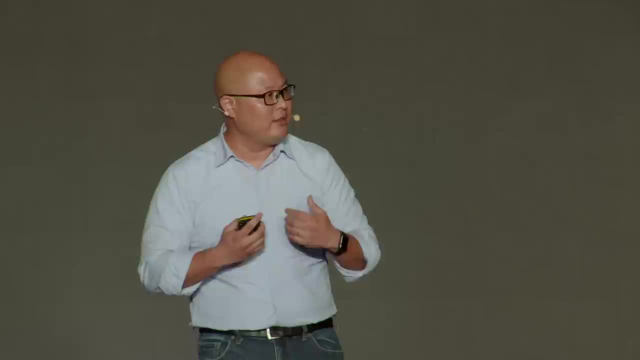 against some logical attack. The second question: how might your perspective be different from that of others? And this forces students to empathize with others. For example, if they're in some kind of debate or something, then this gives students an opportunity to evaluate the grounds of the other side. 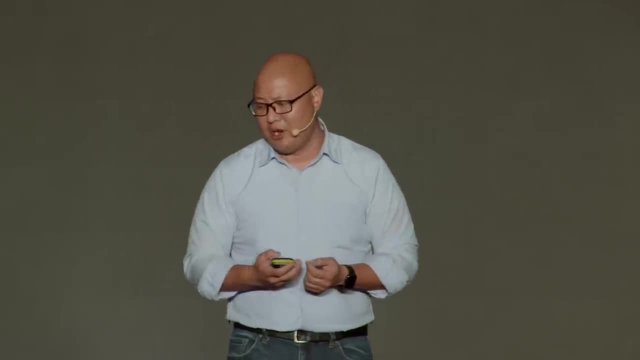 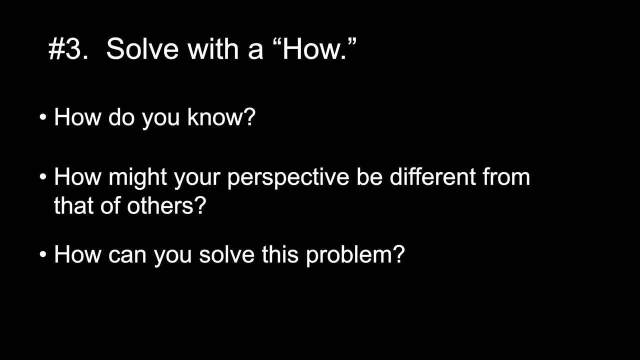 and to consider their needs and maybe to find some common ground. And the final question is: how can you solve this problem? And of course this is kind of the queen mother of all questions. It's huge right, But in doing so, 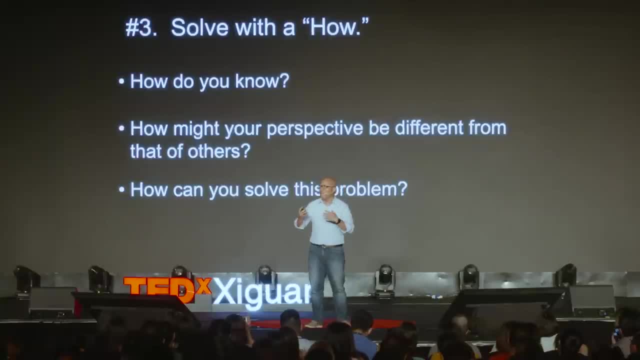 students have to synthesize all of their previous knowledge and be able to figure out how to make this their own and to be able to apply themselves And by taking this huge question and boiling it down into manageable parts, this is a valuable part of the process. 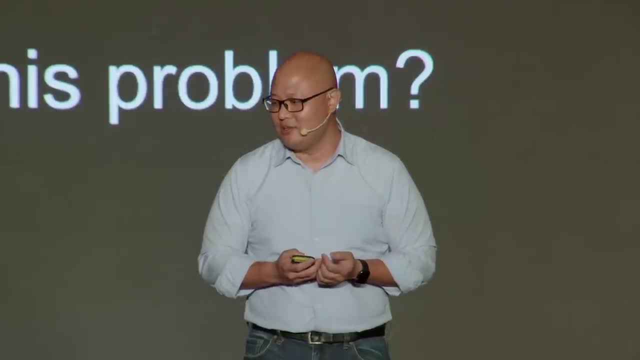 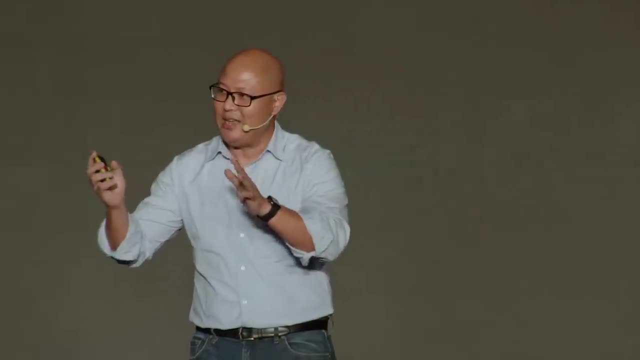 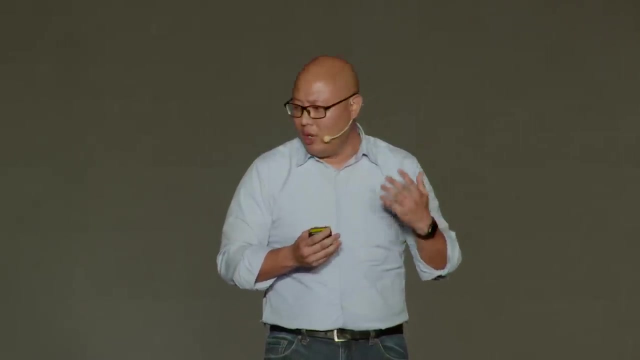 Now, what's the takeaway from all of this? Well, for you students who are listening to this, this is an opportunity for you to extend your learning past the exams. It's an opportunity that will serve you well into the future. In other words, 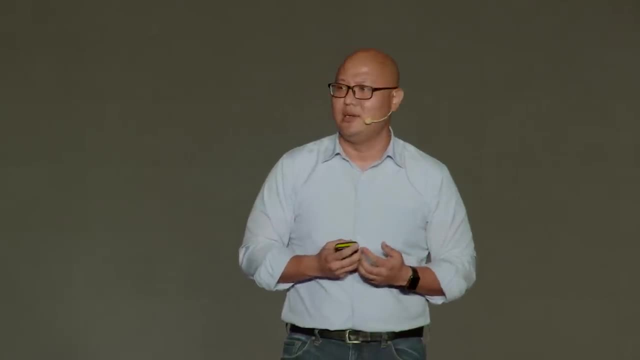 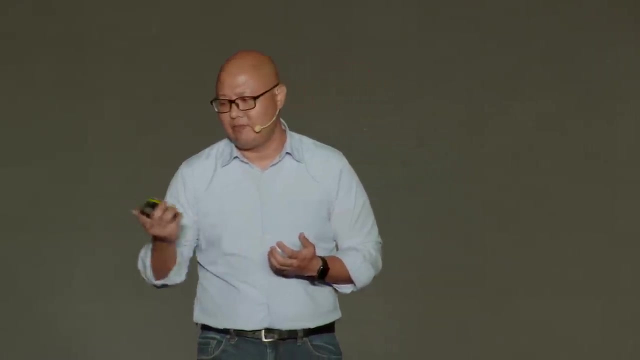 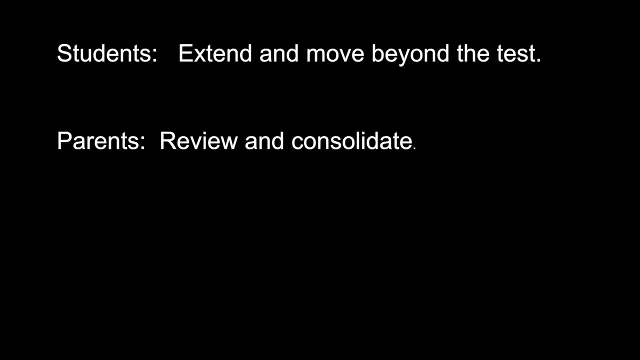 you're not just answering questions for questions' sakes. You're doing it in order to prepare yourselves for the types of uncertainties that you're likely to face. If you're a parent, listening to this. asking better questions is a great way to help your students to review. 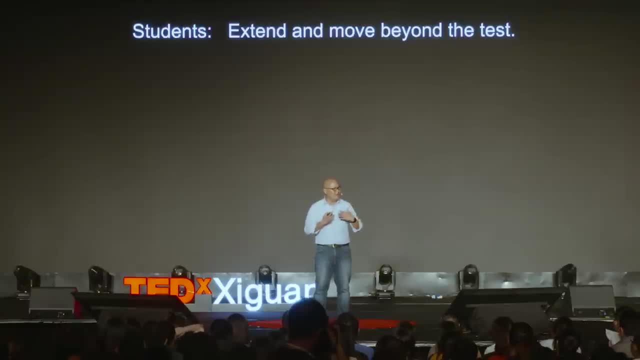 By them having to explain content that maybe they're not as, or maybe that you're not as familiar with. they then have to think about how they're going to put this into sort of digestible pieces for you to be able to understand it. 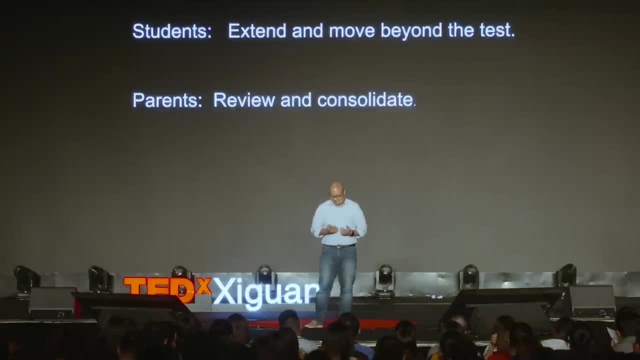 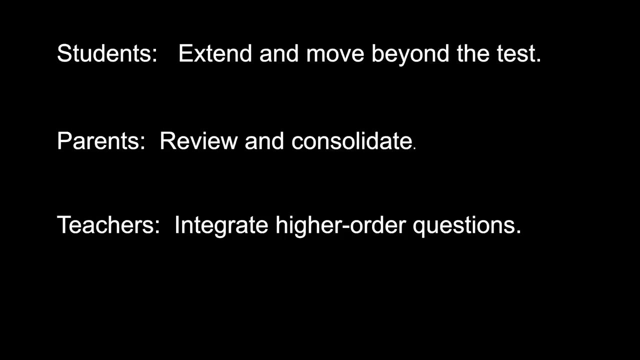 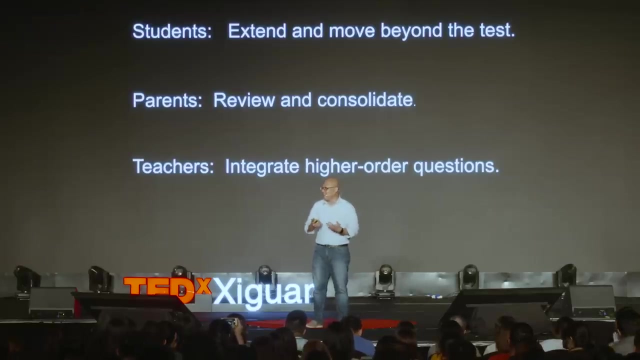 And it's a great way to be able to consolidate learning. If you're a teacher listening to this, think about how you could further integrate higher order questions into your classes And if efficiency is one of the reasons why you're not asking enough higher order questions. 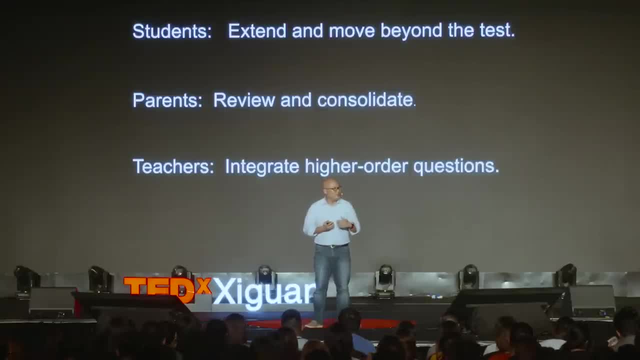 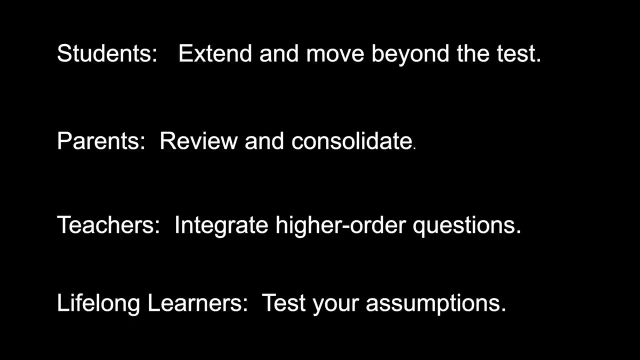 then evaluate the sort of activities you do with your students in class And if they don't go toward the goal of advancing critical thinking and creativity, then think about whether or not these activities are truly relevant And if you're a lifelong learner, ask yourself these questions. 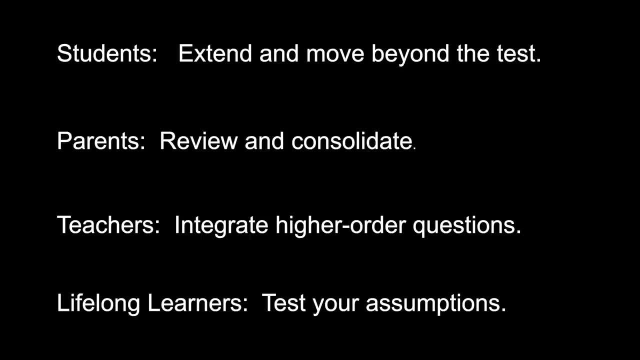 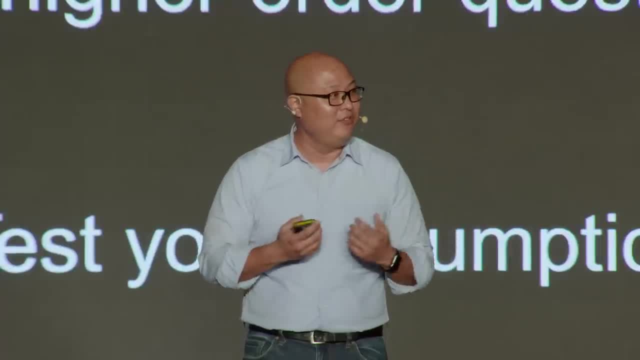 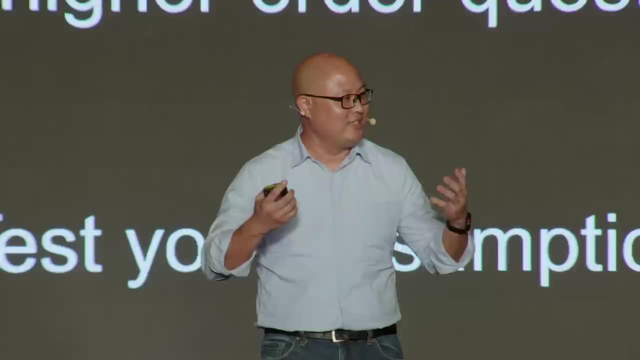 in order to test your assumptions about what you think you already know. At the very least, you'll be able to empathize with the other side and to possibly find some common ground. Now, you know, it's naive for us to think and for me to stand up here and to say that 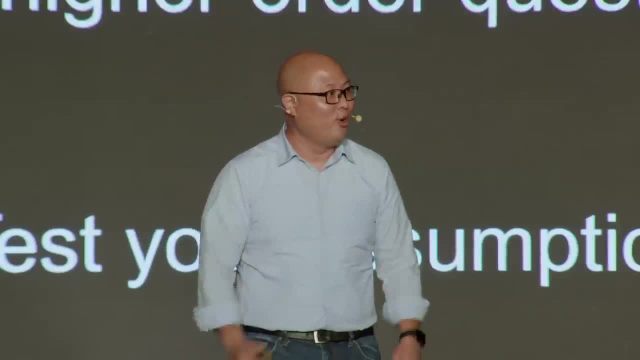 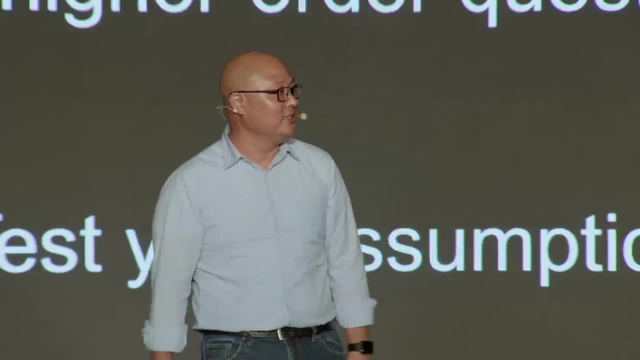 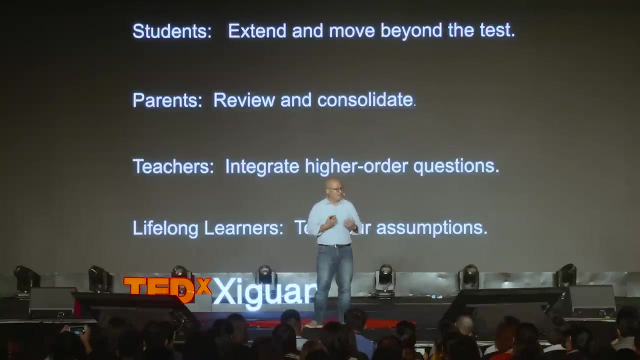 you know, just by asking a few more how questions, or a few more why questions, that this is going to be enough to create the next generation of great innovators and critical thinkers. After all, it takes a kind of group effort, one in which schools collaborate with teachers.